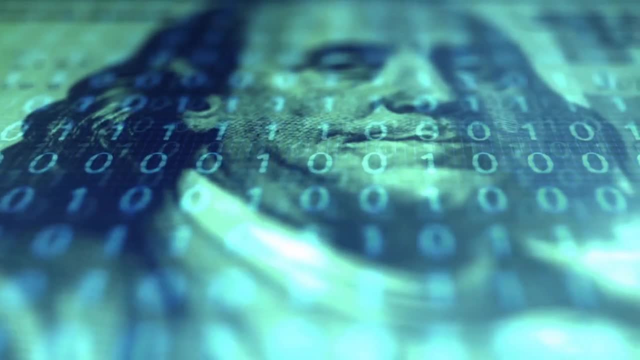 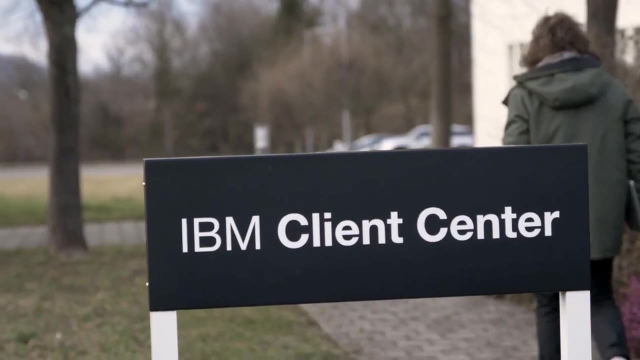 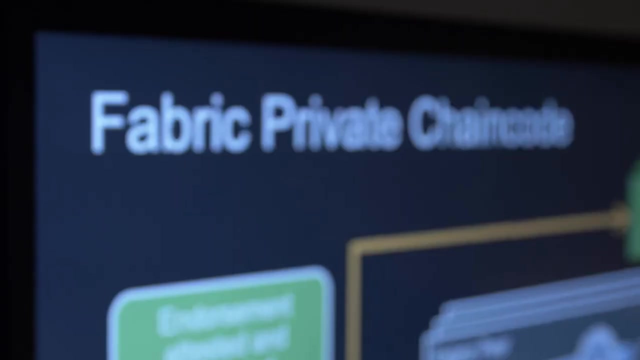 kind of auction we are talking about billions of dollars so the temptation to try to gain the system can be very high recognizing this challenge and starting from separate efforts at IBM research and Intel labs the two companies decided to join forces to create fabric private 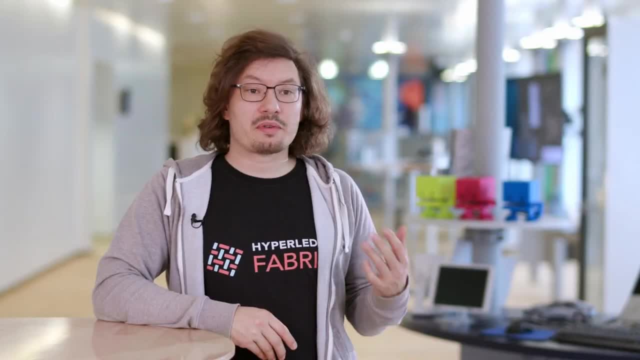 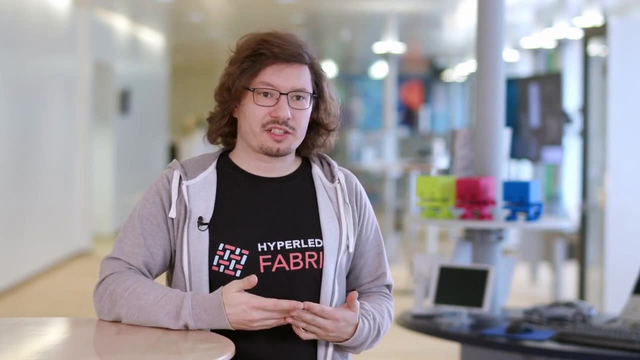 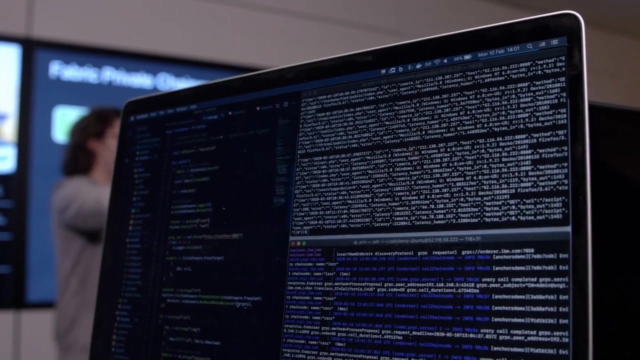 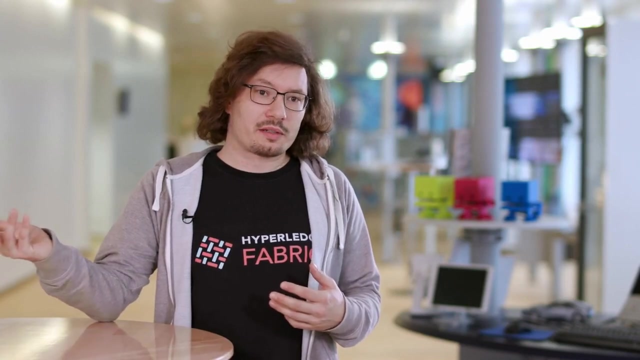 chain code fabric private chain code is a framework for the use of wireless technology for the hyperledger fabric blockchain to develop and run smart contracts using Intel SGX Intel SGX is a trusted execution environment that allows a program to remain encrypted while running it's not even observable by the system administrator or any other privileged software 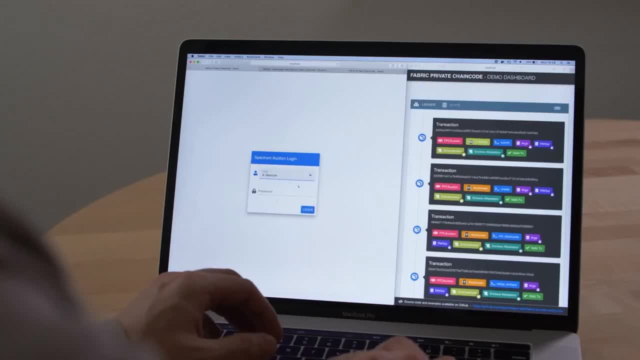 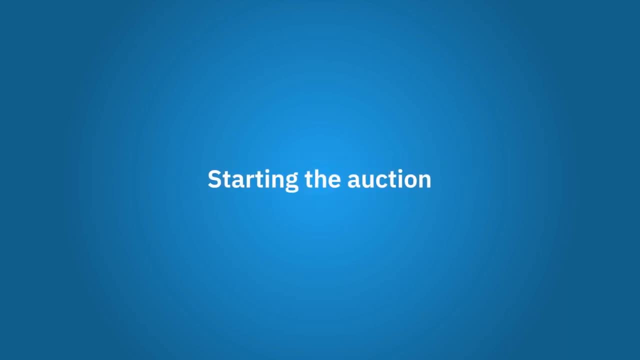 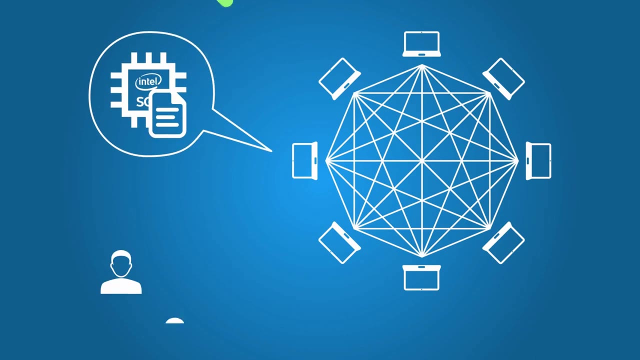 this solution enables confidentiality let's have a look at a demo of a spectrum auction to begin the auction the auctioneer deploys the auction chain code on the network participants can then verify that the correct chain code has been deployed and has not been 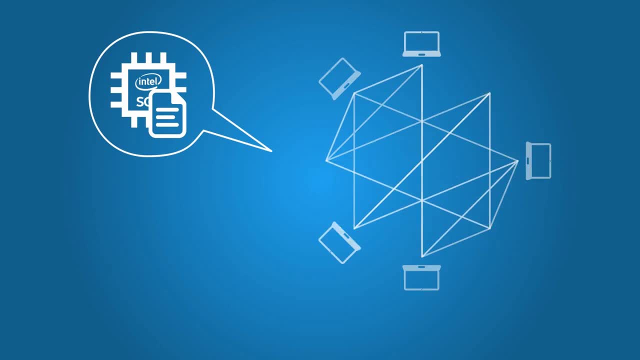 tampered with once the chain code is up and running the auctioneer sets up the auction 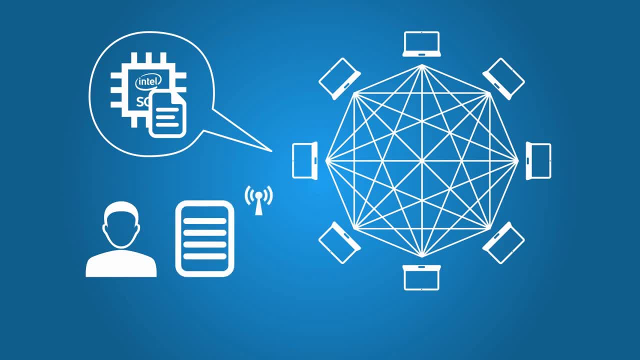 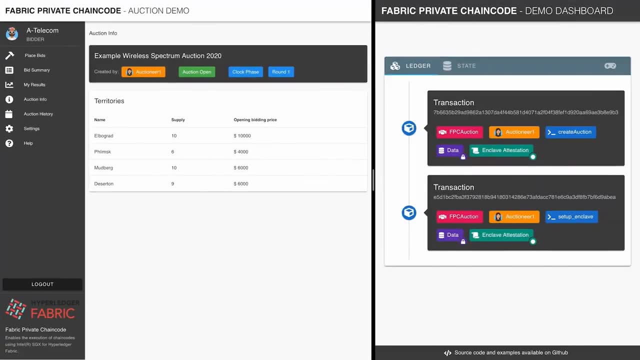 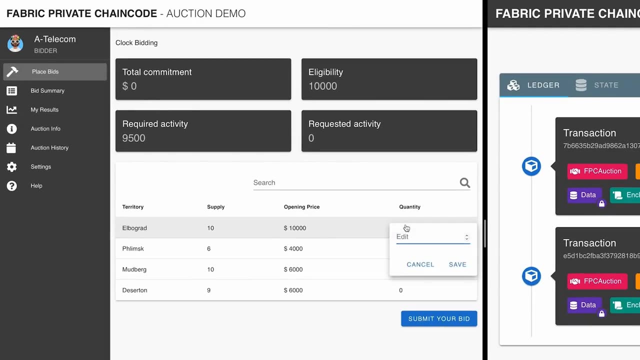 details including the available spectrum licenses and the participants now it's time for the bidders to enter their first bids and submit them as transactions once the bid is created the user submits their bid to the chain code 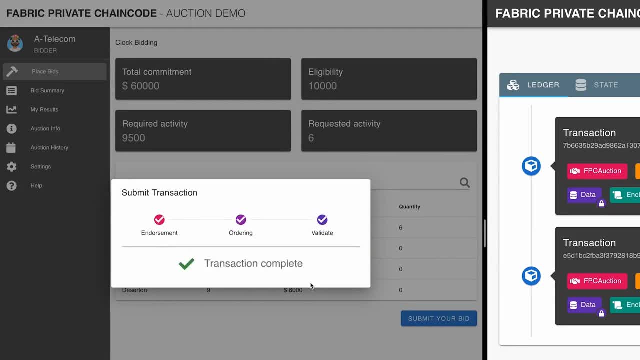 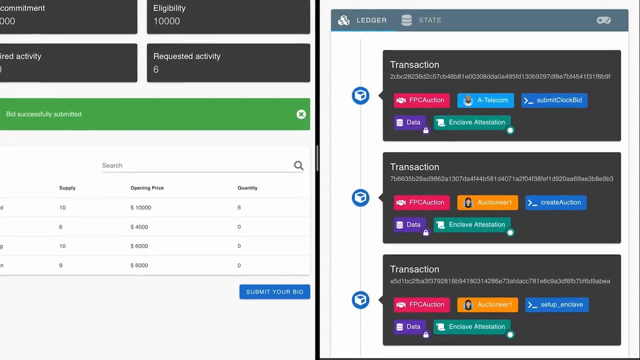 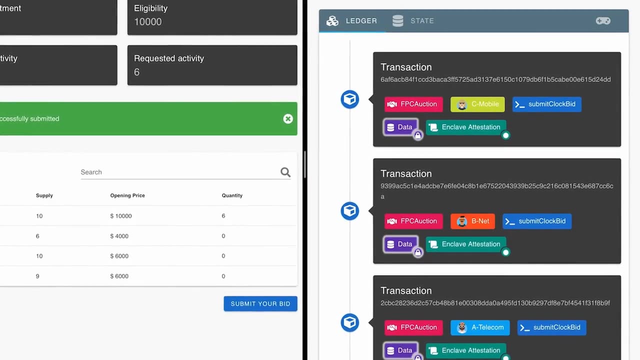 once the transaction is committed to the blockchain it can be seen in the viewer it is encrypted in a way that neither the other bidders nor the auctioneer can read the contents in the meantime the other bidders are also placing their bids The content of their bids cannot be seen. 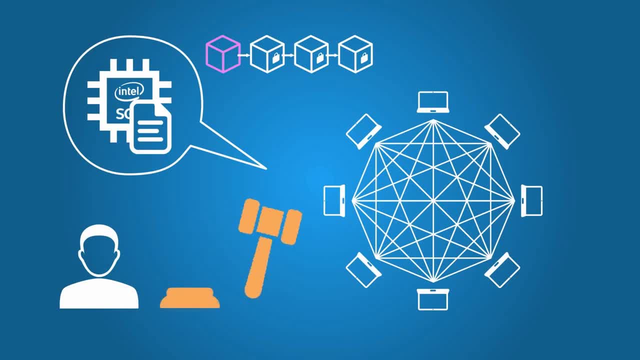 Now, the auctioneer closes the auction. The chaincode reads the bids from the ledger, decrypts them, and announces the results in public. 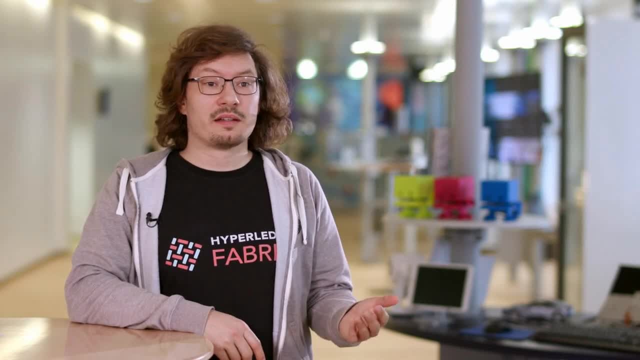 Fabric Private Chaincode is a new way to run smart contracts on Hyperledger Fabric. 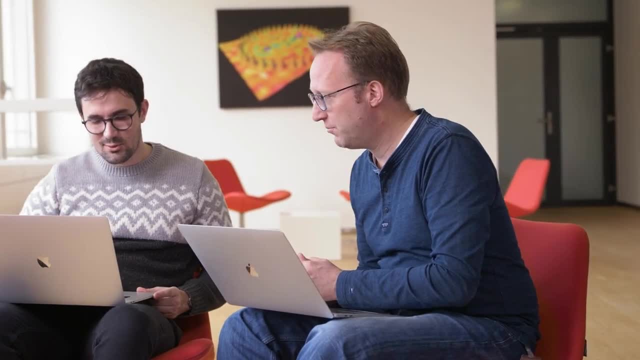 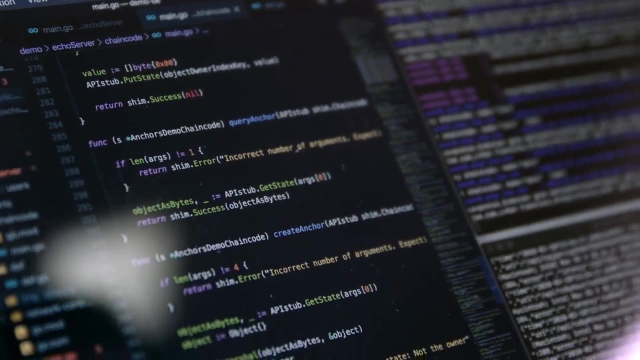 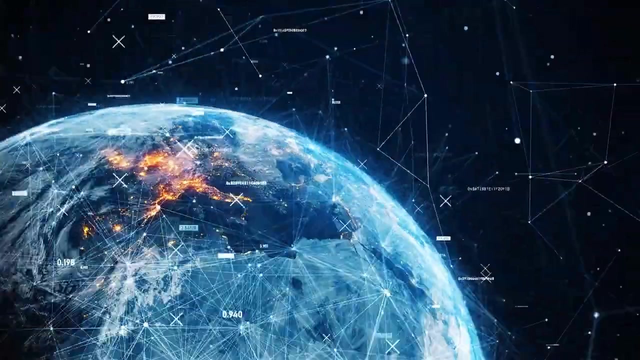 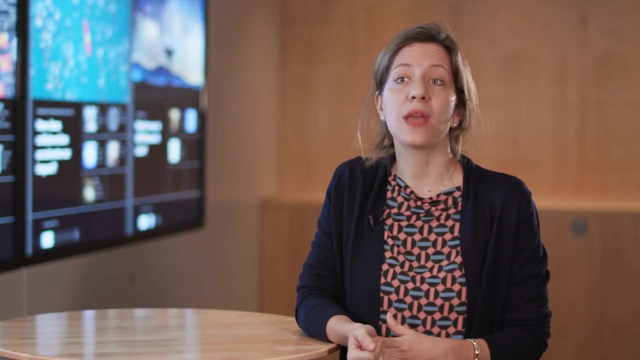 Our design and the use of Intel SGX enable a new model of trust otherwise not possible with Hyperledger Fabric. So, in many real-world situations and scenarios like this one, this private auction, we expect Fabric Private Chaincode to bring value by reducing the capability and eliminating the incentives to game the system. 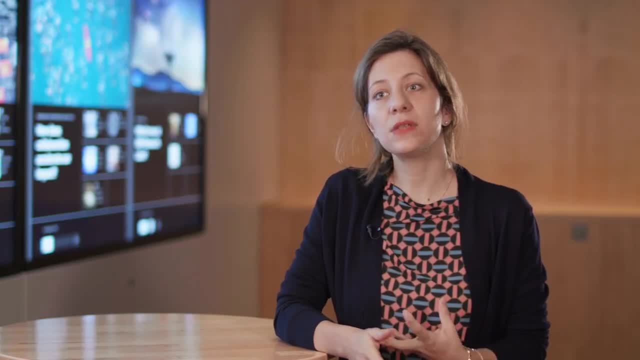 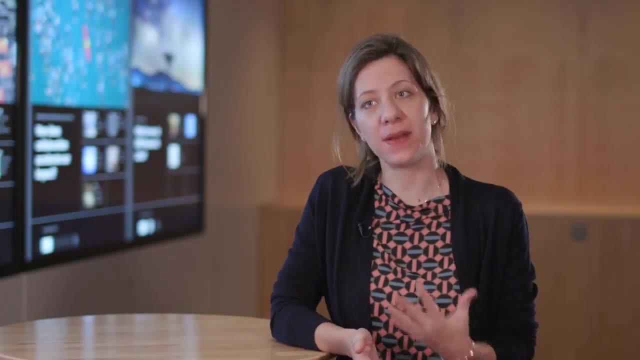 So, with this new technology, one can really strengthen the trust to the system, and by doing so, one can reduce the costs associated to maintaining highly expensive security measures, insurance, and legal fees. 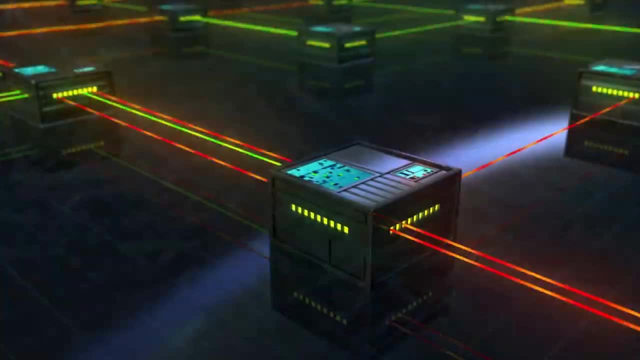 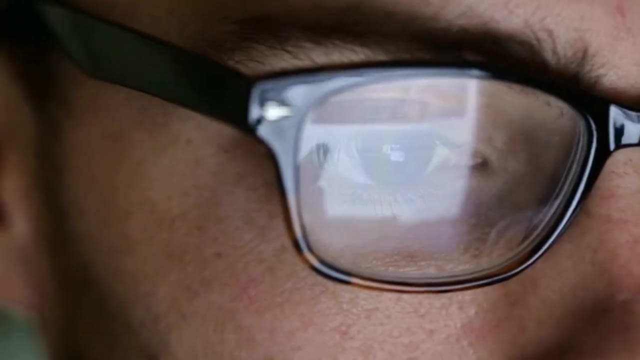 IBM and Intel believe that, in the future, Fabric Private Chaincode can facilitate the adoption of trusted execution environments and move beyond specific high-stake use cases towards the widespread use in blockchain applications, similarly to what HTTPS did. 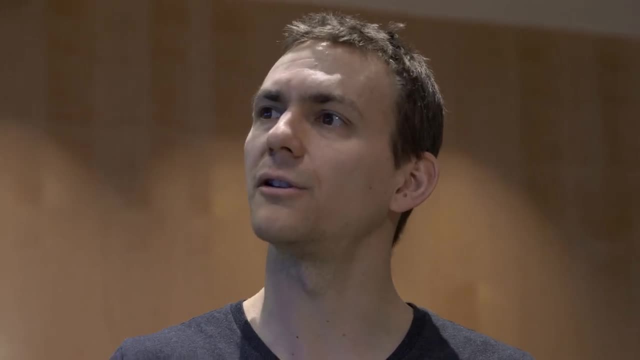 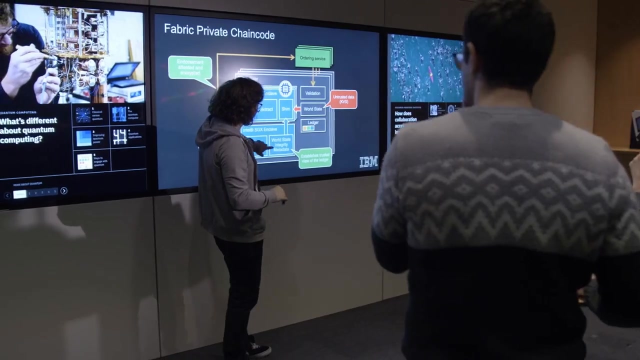 Fabric Private Chaincode is an open-source project supported by the Hyperledger community. It is now ready to be considered for pilot deployments of real workloads. Check out our project on GitHub to learn more. 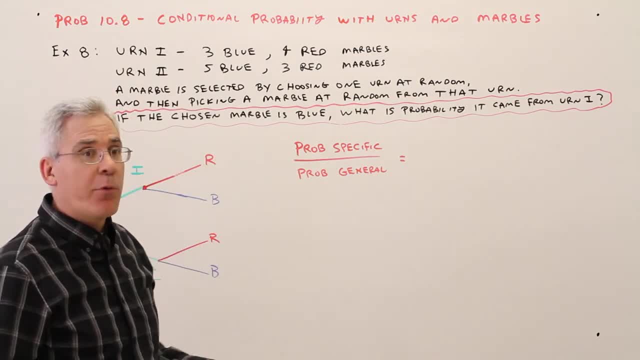 Welcome to Probability Video 10.8, Conditional Probability with Urns and Marbles. Alright, here's Example 8.. Urn 1 has 3 blue and 4 red marbles. Urn 2 has 5 blue and 3 red marbles. 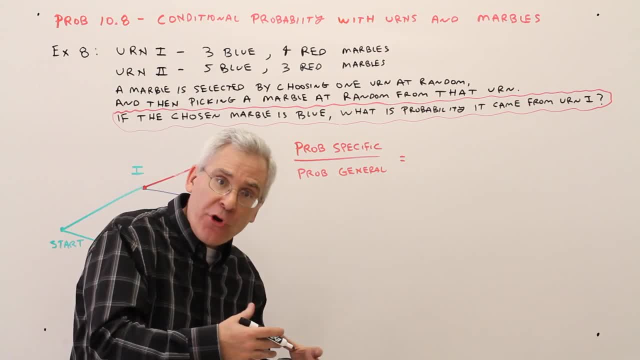 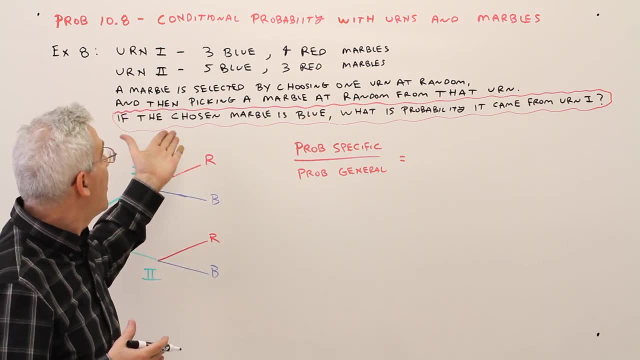 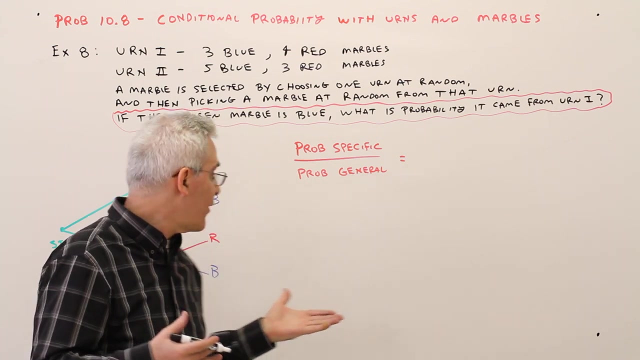 A marble is selected by first choosing an urn at random and then, within that urn, selecting a marble. Alright, the question is: if the chosen marble is blue, what's the probability that it came from urn 1? Alright, so for problems like this, I like to start with a tree diagram.